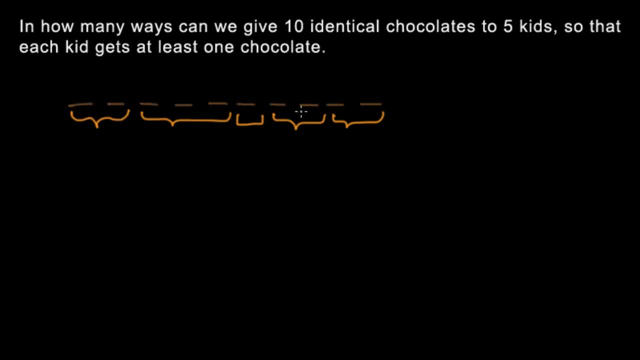 But then the first kid could also get 1, 3, 2, 2, 2 or something, And it's really hard to count all of them because there are just so many ways you could achieve this. So we're going to attack this problem in a different way. 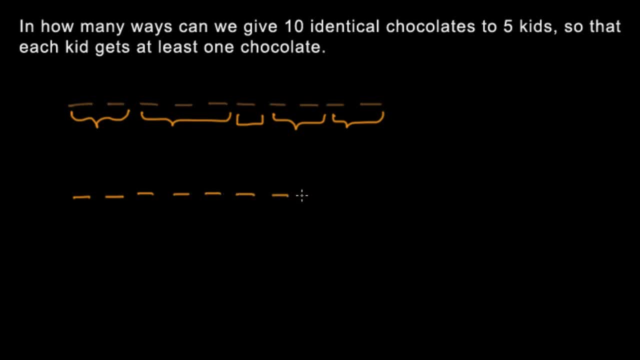 So you have 10 chocolates And say that by putting in a divider like this, the first kid gets the number of chocolates before the divider To the left, the first kid would get 2 chocolates. Similarly, if we put another divider right here, 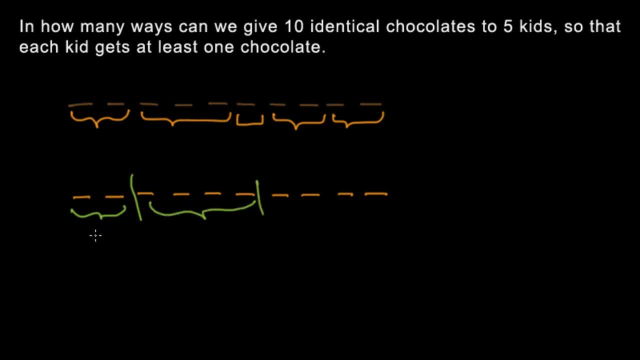 the second kid would get 4 chocolates, And again the third child would get 1.. And the fourth would get, for example, the fourth child would get 2 and the fifth would get 1.. So we can think of this problem as: 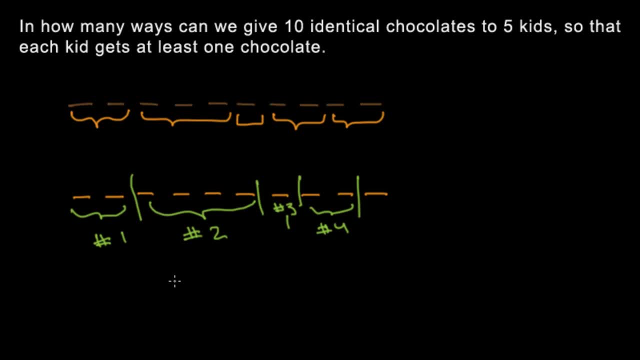 the number of arrangements of chocolates with 4 dividers. So this is simply just how many number of ways can we arrange again: 10 chocolates and 4 ticks. So we can rewrite this as total number of items, which is number of places you can put the ticks in is 9. 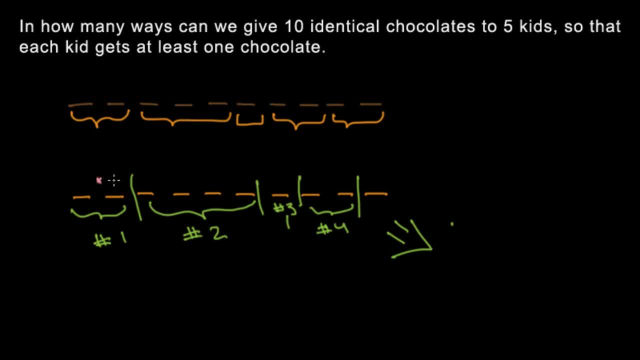 because you can put either here, here, here, here or here, And you can't put the dividers here or here, because each kid should have at least 1 chocolate And 1 kid can't have 10 chocolates all at once. 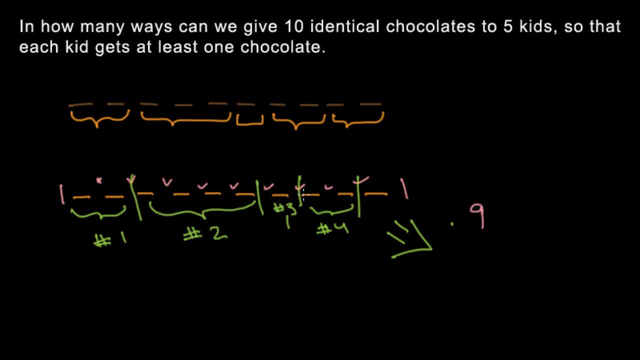 So you have 9 spots to put the dividers in And you have to give it to 5 different kids, So that's 4 dividers And you have to choose places to put 4 dividers in the 9 spots. 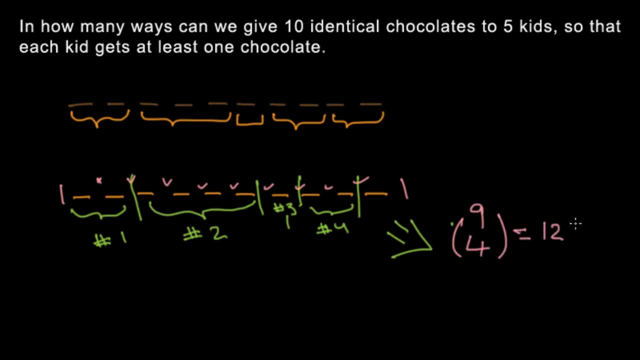 which is 126.. This is a distribution problem where you convert the number of indistinguishable items into distinguishable boxes. So try coming up with a formula where you have n identical items, where you have to give it to k people, and try to see if you got the concept.